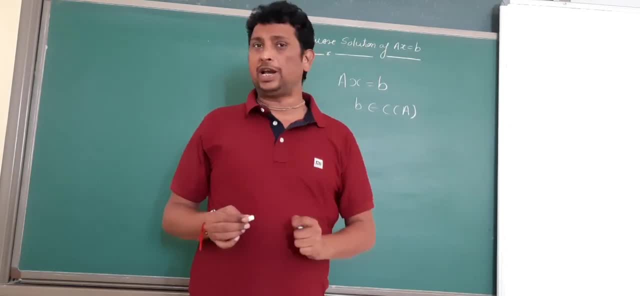 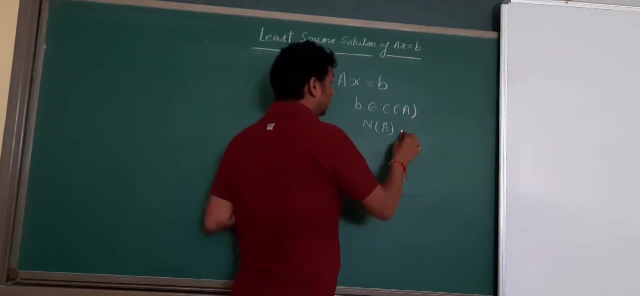 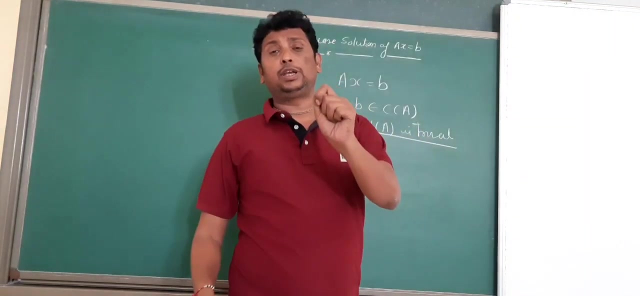 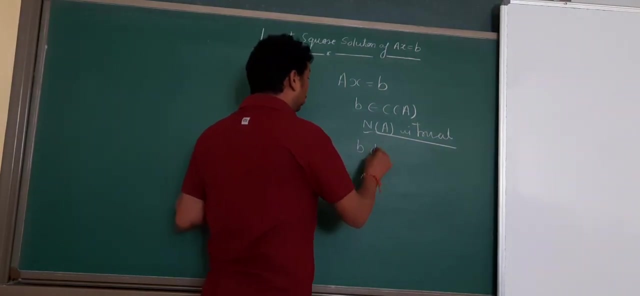 But how many? Is it unique or infinite? Then unique exists when we calculate null space of a and it is trivial. If null space of a is trivial, we say solution is unique. But what happens if b does not belongs to column space of a? 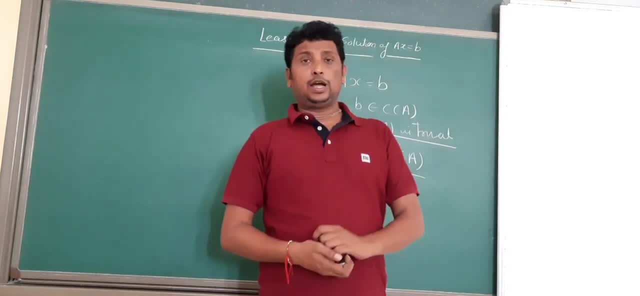 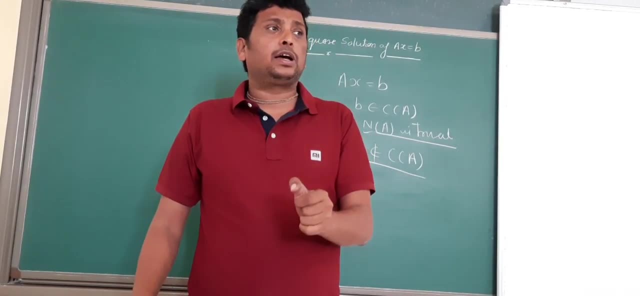 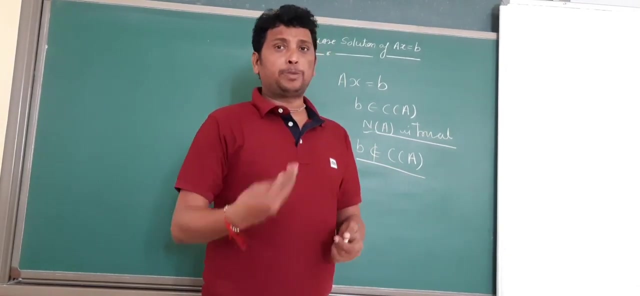 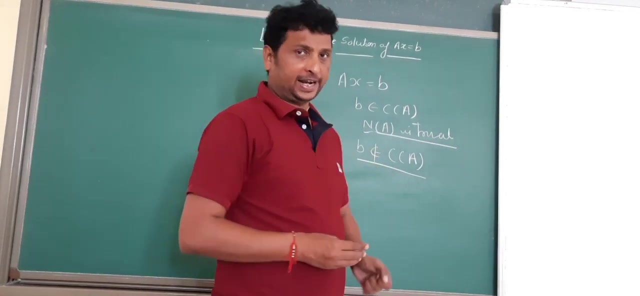 In this case, system is inconsistent and then concept came. It means we have inconsistent system, So we are going to calculate approximate solution. That's why it will come in terms, sometimes in form of numerical approximation technique. So it means what we are going to do. 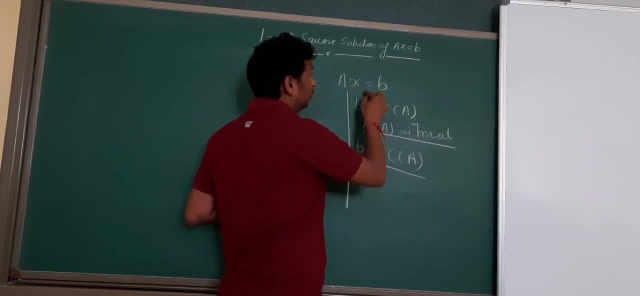 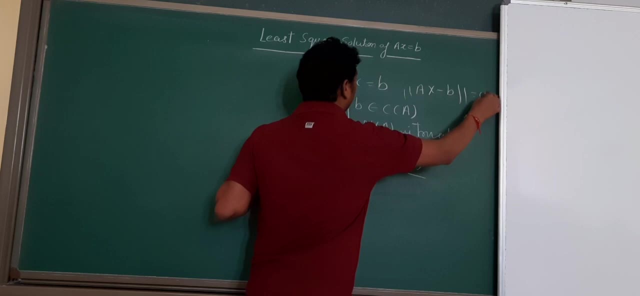 We are going to actually solution of this system is we are getting ax minus b. So we are going to actually solution of this system is we are getting ax minus b. So it means what we are going to do. We are getting ax minus b closely to zero. 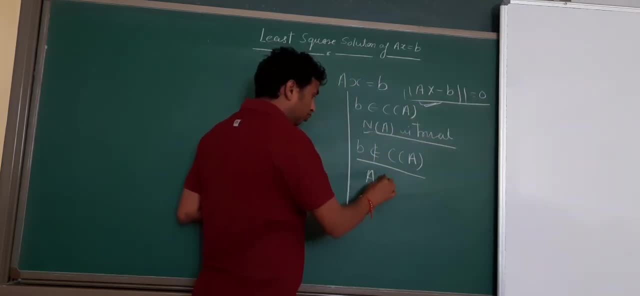 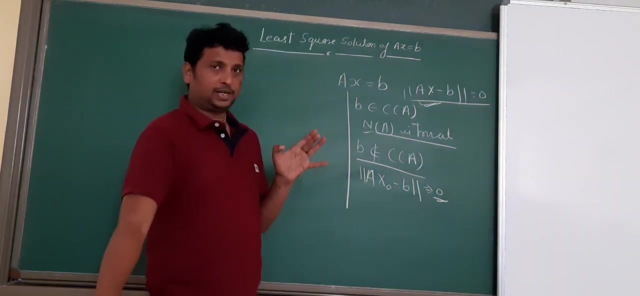 Okay, so same type here We are going to find that x0, such that a x minus b approaches to zero. It will approach to zero, That x0 we are going to calculate, and that x0 is known as least square solution. Understand: 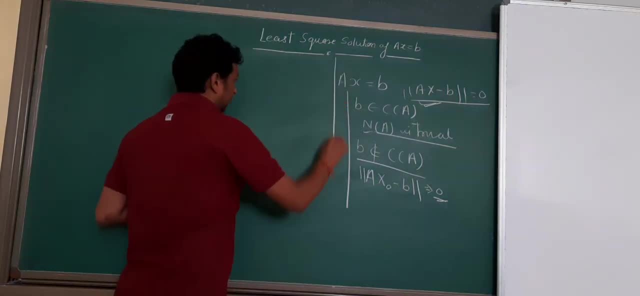 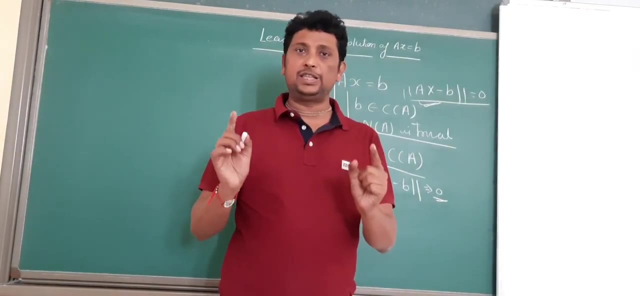 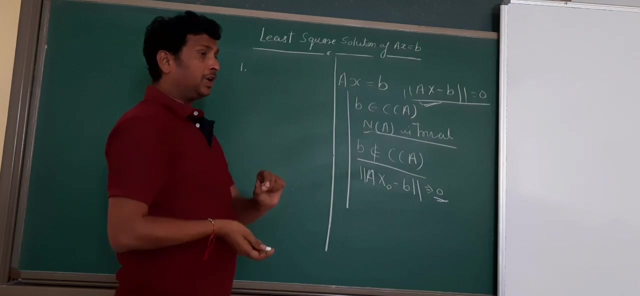 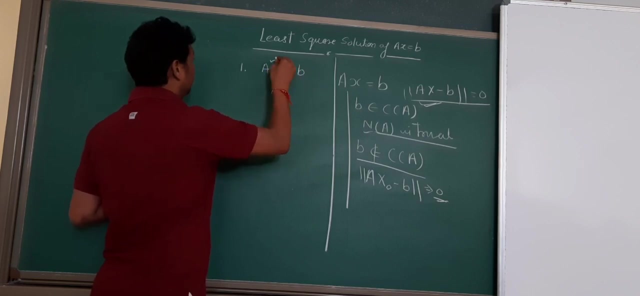 okay now how we calculate. there are so many methods which are lengthy, but one method, which i am going to explain it easy and easily, you can do, and that is first step, is very simple. whatever matrix given, a system given, write in a matrix form, a, x is equal to b, which easily you. 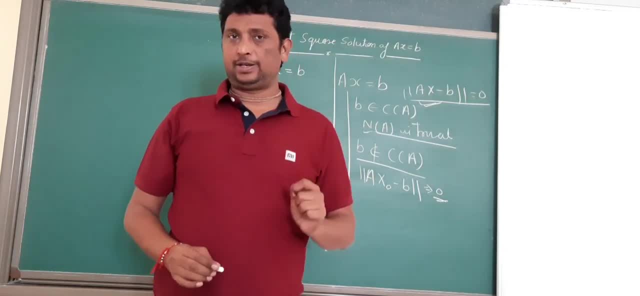 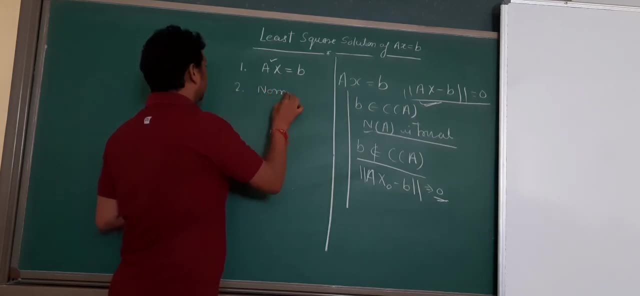 can write. okay, once you retain in a matrix form, then your second step is write normal equation, normal equation. what is normal equation? it's very simple: a transpose into a, x is equal to a transpose into b, which you can write easily because a you know, b you know. 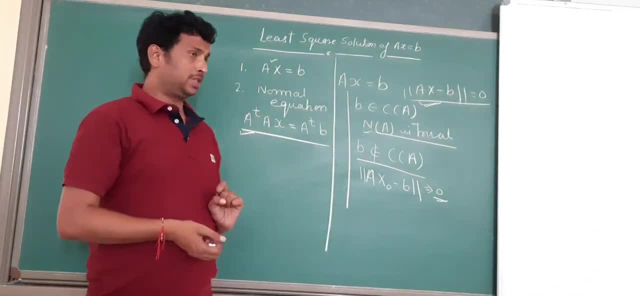 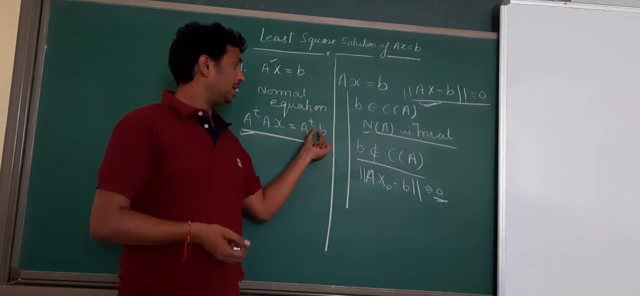 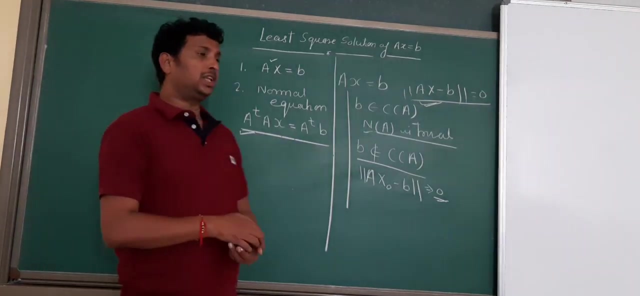 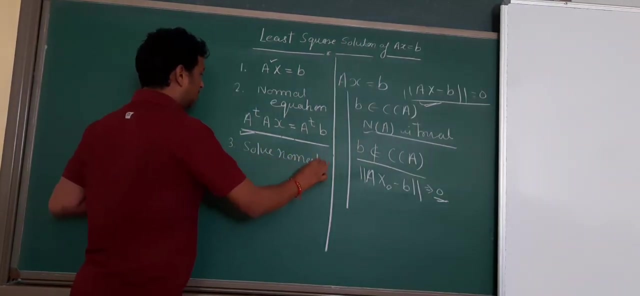 a you know, then you can calculate a transpose easily. then find out a transpose into a correct. and find out a transpose into b, then write this equation. once we have this equation, let's solve that equation. solve normal equation. how? using using gauss elimination means making this system. 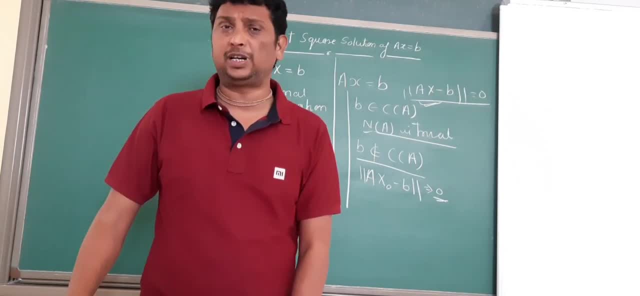 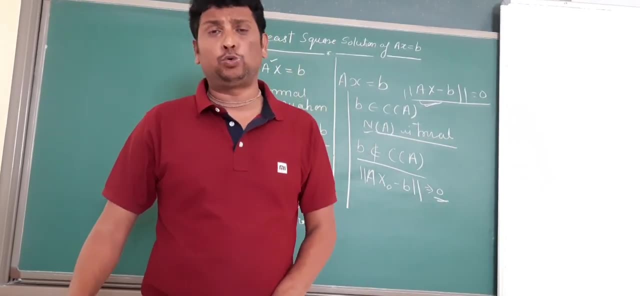 in upper triangle form. you know what was elimination method. we first we write argument matrix and then we go for to reduce that system into upper triangular matrix form and And then we write again in a system equation form and we calculate by a bad substitution. That is Gauss elimination method. 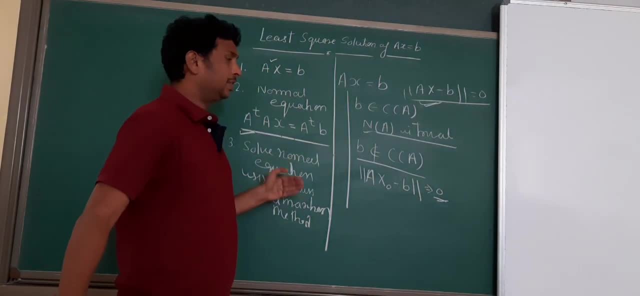 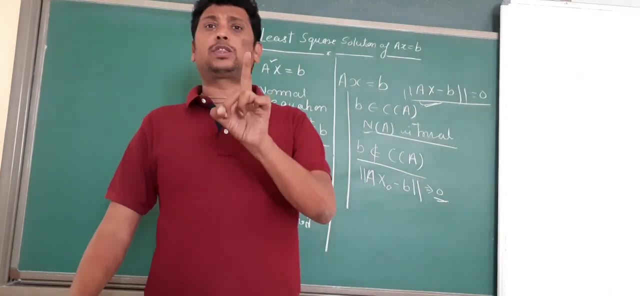 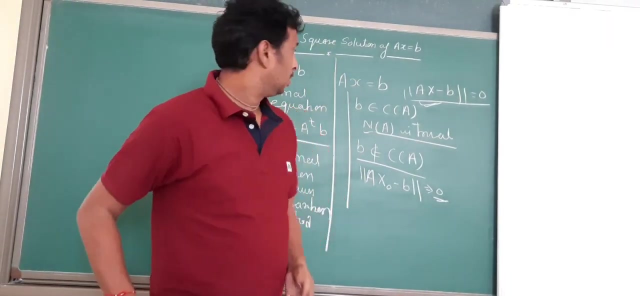 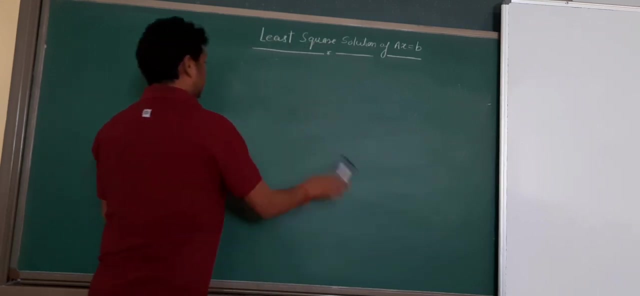 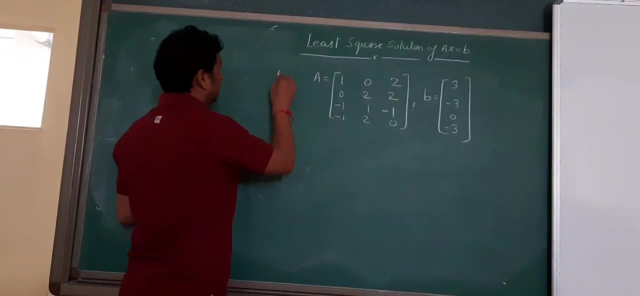 So once you find out solution of this system equation, that is, your least square solution, Means solution of normal equation is known as least square solution. So now we are going to take one example and we will do it. We are going to solve this example. 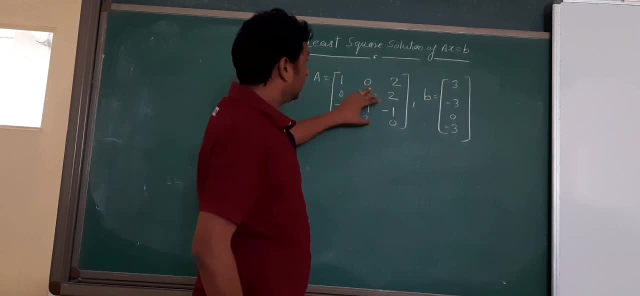 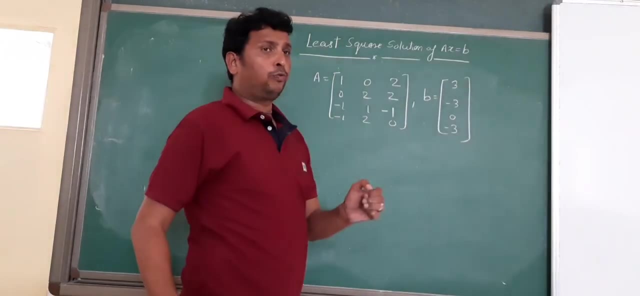 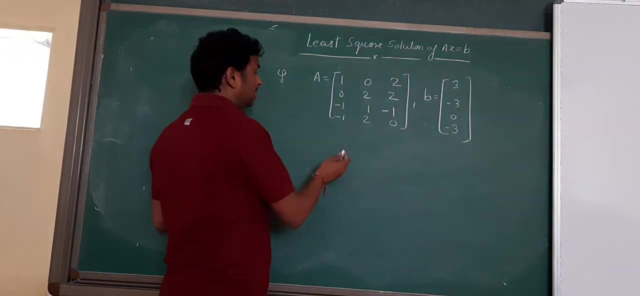 The example is: A is given this and B is given this Means system of equation given in matrix form And they ask to find out least square solution, whatever is there for this system of equation. So how we do, What is first step? 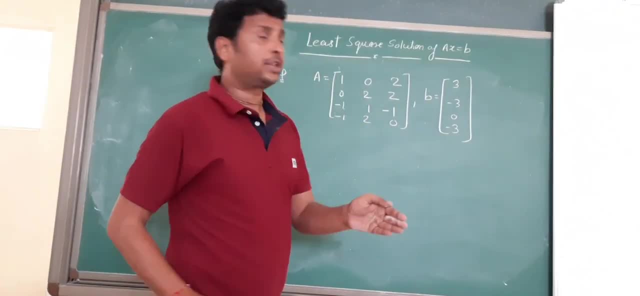 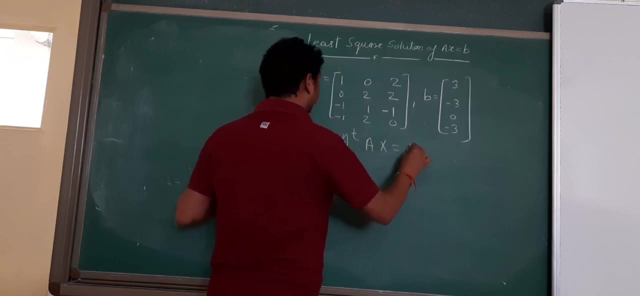 Write in a matrix From that already given. So what is second step? We have to write normal equation. What is normal equation? A transpose of A into X is equal to A transpose into B. So A given. So first we calculate A transpose into A. 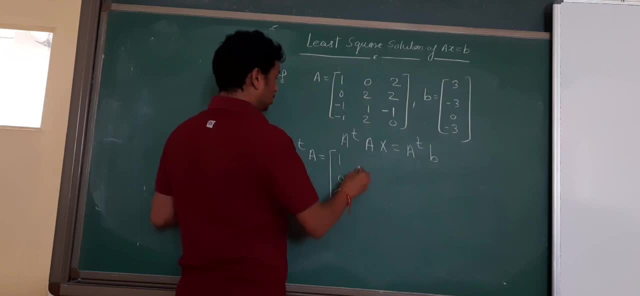 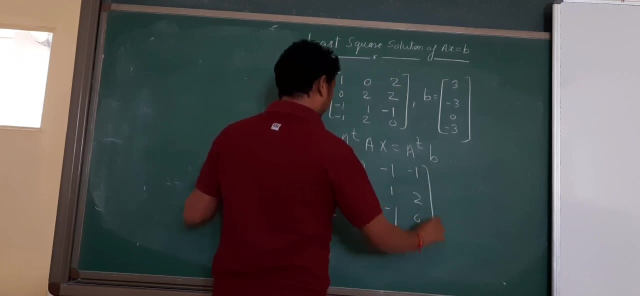 What is A transpose? 1, 0, 2. 0, 2, 2.. Minus 1, 1.. Minus 1.. Minus 1, 2, 0.. And what is A? 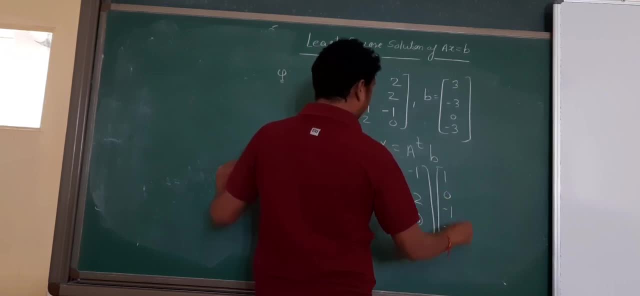 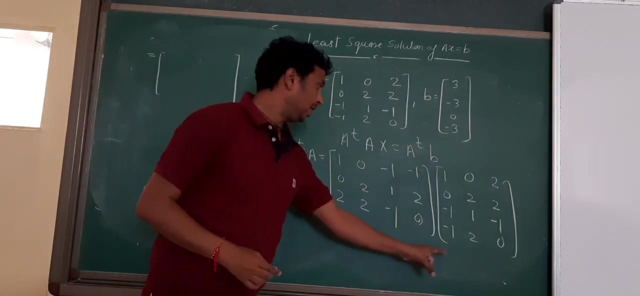 A given 1, 0.. Minus 1, minus 1. 0, 2, 1, 2.. 2, 2, minus 1, 0.. What is the value? So value is A. transpose into A. 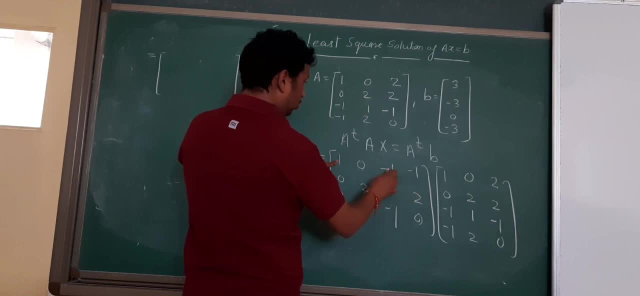 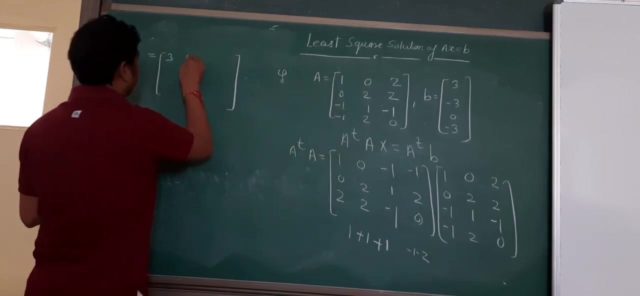 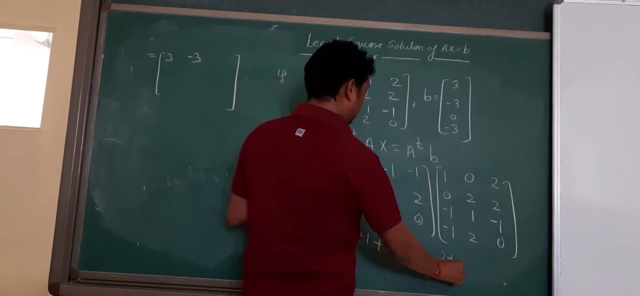 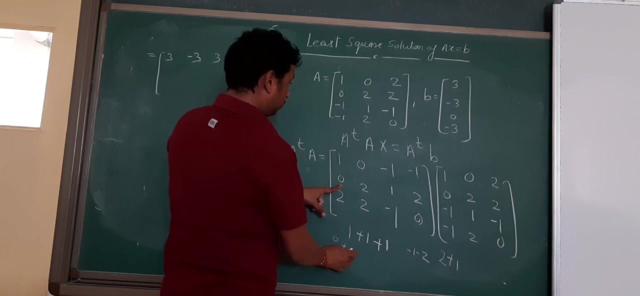 What we get: 1, 0, 1, 1, 3.. Second Second: 0, 0, minus 1, minus 2, minus 3, 2, 0, 1, 0, 3, similarly second: 0, 0, minus. 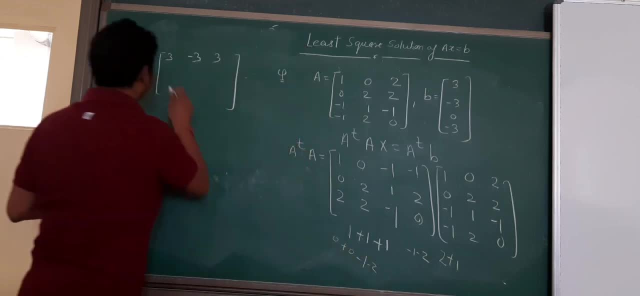 1, minus 2, minus 3.. Then 0, 0.. 0, 0, minus 1, minus 2, minus 3.. Then 0, 0, 4.. 3, 4.. 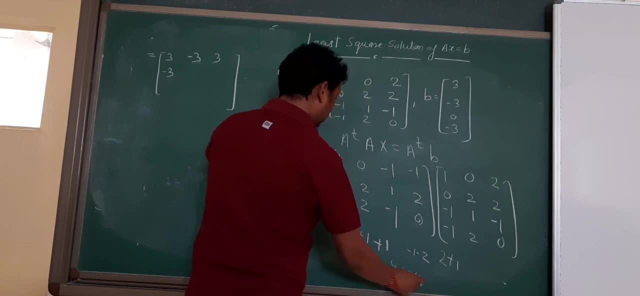 1,, 1,, 2,, 3,, 4.. 1, 4,, 1,, 2,, 4,, 3,, 3,, 4, 4.. We named: 3. 3, 1,, 1,, 2,, 4,, 5,, 5,, 6,, 6,, 7,, 8.. 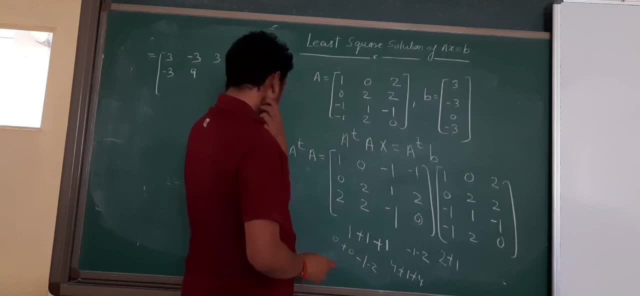 3, 1, 1, 2,, 4,, 5,, 6, 7, 8.. 1, 1, 1, 2, 9.. A a number綳 3, a numberwe treated: 0, 1, 2 free. 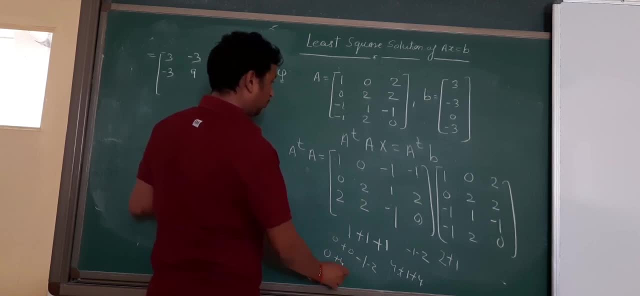 A third: 0, no 0, 1, 3.. 2, 1, 1, 2, 0, minus 1, 0, 4. Minus 1, 0.. 0, 3.. 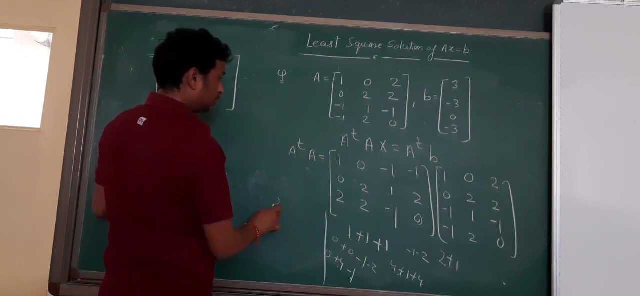 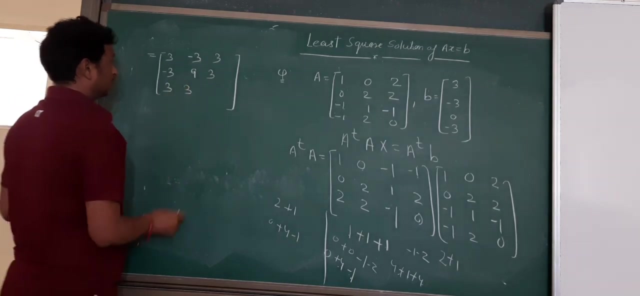 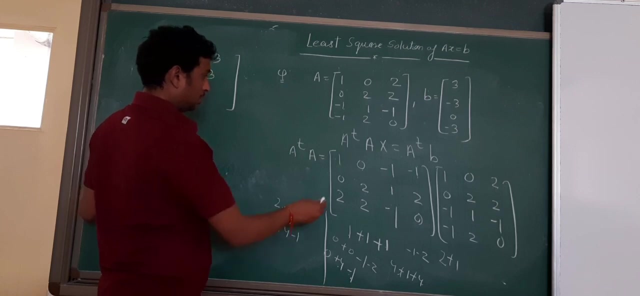 3, 2, 1, 2.. Did you catch my mind? 3, 1, 1, 2.. 1,2,3,4,5,6,7,8,9,10. 1,2,3,4,5,6,7,8,9,10. 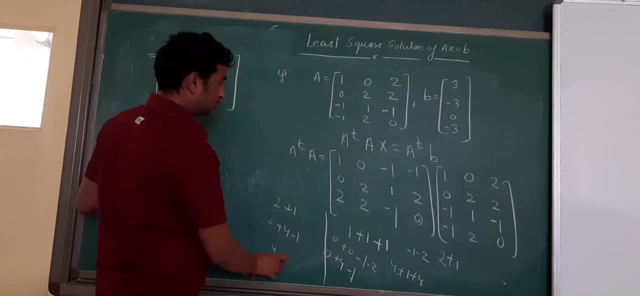 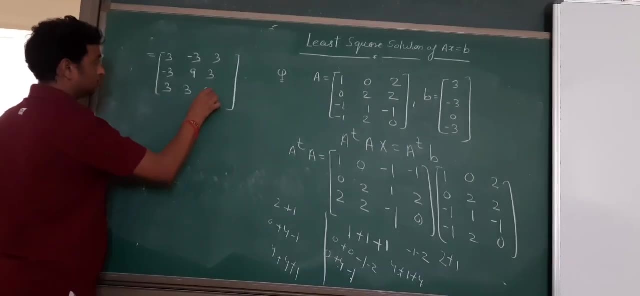 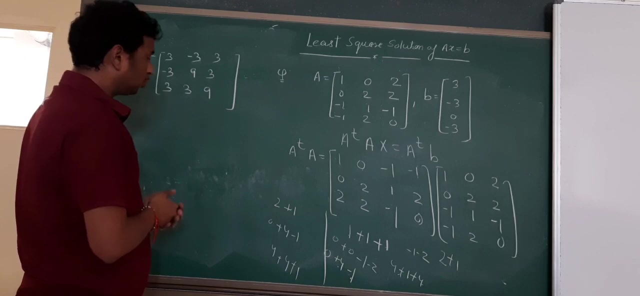 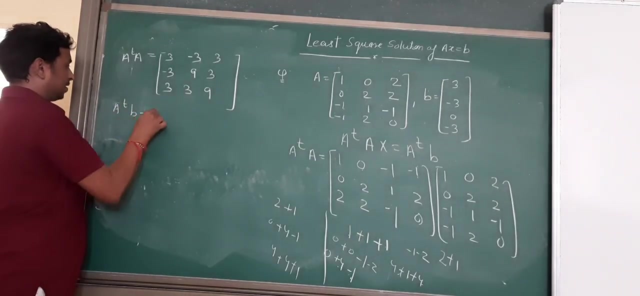 1,2,3,4,5,6,7,8,9,10. 1,2,3,4,5,6,7,8,9,10, 1,2,3,4,5,6,7,8,9,10. 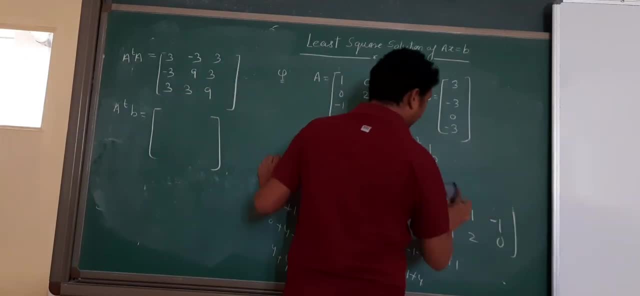 1,2,3,4,5,6,7,8,9,10. 1,2,3,4,5,6,7,8,9,10, 1,2,3,4,5,6,7,8,9,10. 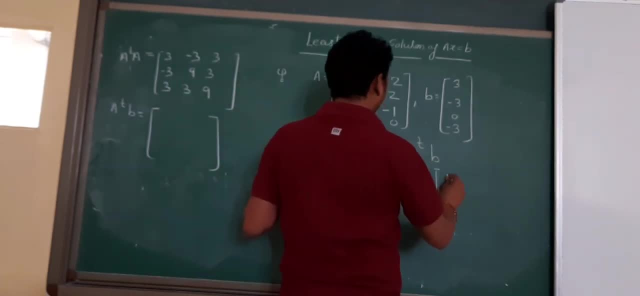 1,2,3,4,5,6,7,8,9,10. 1,2,3,4,5,6,7,8,9,10, 1,2,3,4,5,6,7,8,9,10. 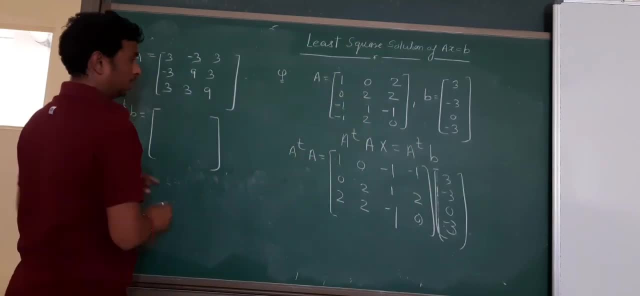 1,2,3,4,5,6,7,8,9,10. 1,2,3,4,5,6,7,8,9,10, 1,2,3,4,5,6,7,8,9,10. 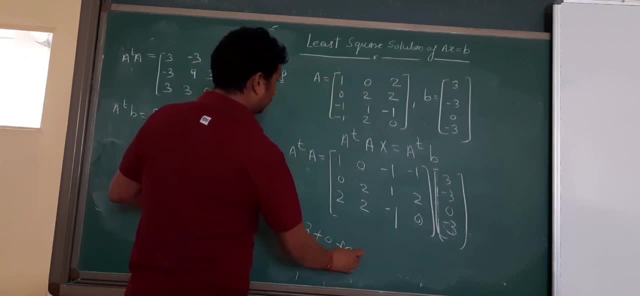 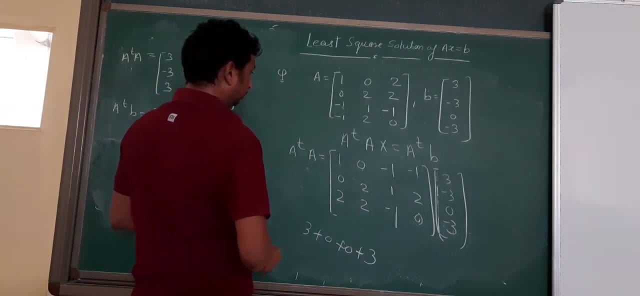 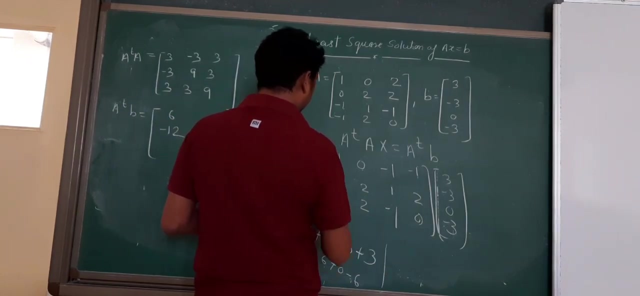 1,2,3,4,5,6,7,8,9,10, 0, plus 3, 6, then 0, minus 6, 0, minus 6, minus 4,, then 6, minus 6, 0, minus 6,. 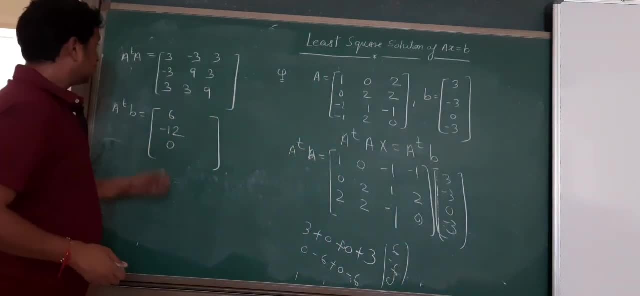 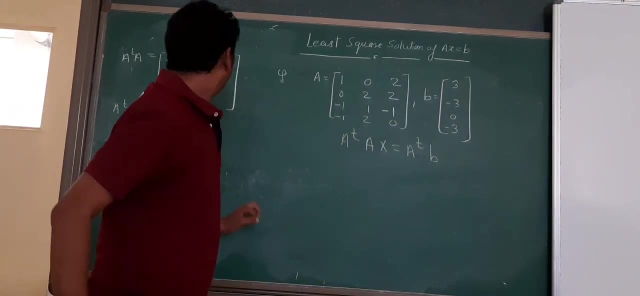 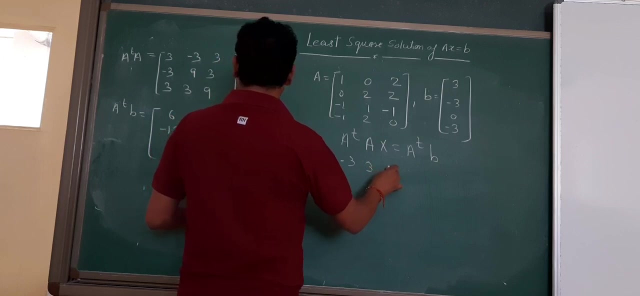 0,. this is the data. what is it to be so what is the normal equation? normal equation becomes 3, minus 3, 3, minus 3, 9, 3, 3, 3, 9, into x means x1, x2, x3, x3, x3, x3, x3,. 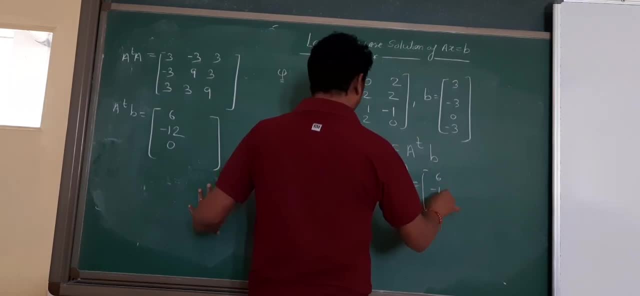 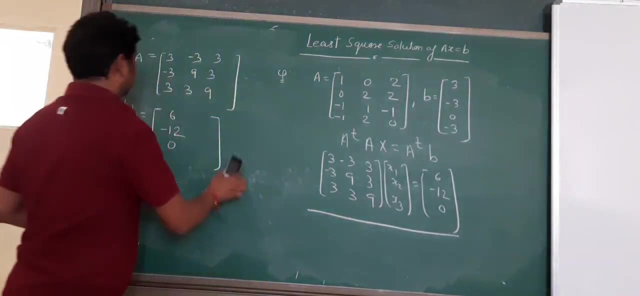 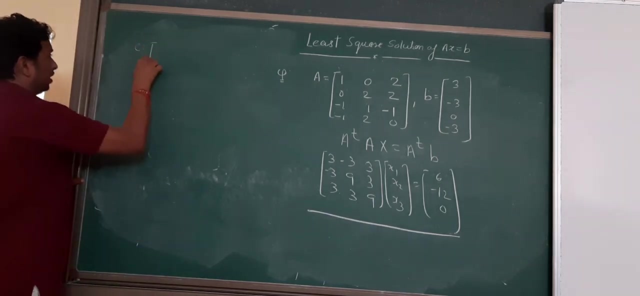 and what is the probability? 6 minus 0, 0,. so now we have to solve this system of equations. so how we solve? we write all the interminables and that is what. 3, minus. 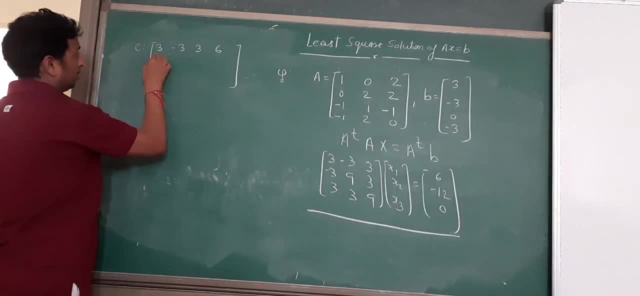 3,, 3, 6,, then minus 3, 9,, 3, 12,, then 3, minus 3, 9, 3, 12,, then 3, minus 3, 9, 3,. 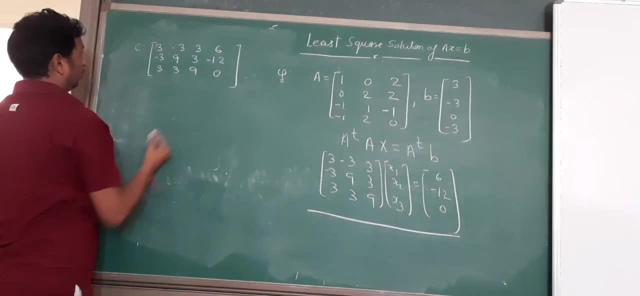 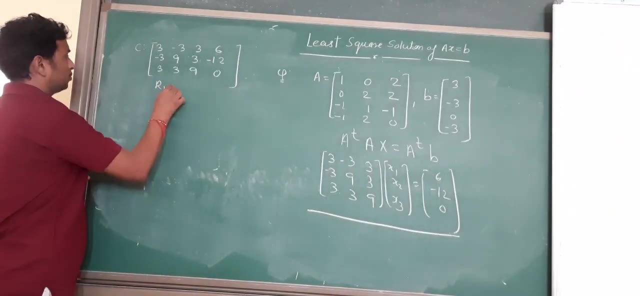 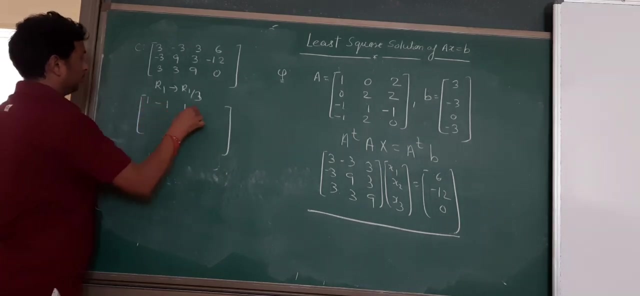 3, 9, 0,. now we reduce this system, system into upper tabular matrix. and how? so divide R1,, divide it to R1, R3, what do you get? 1, minus 1, minus 2, instead, and this is minus. 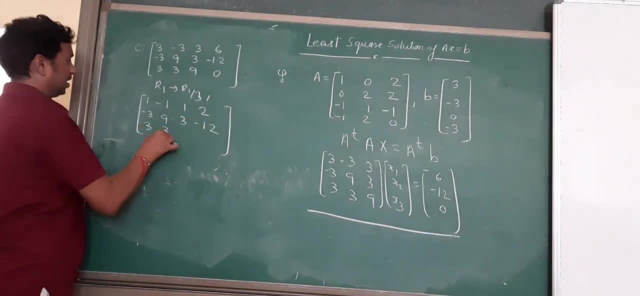 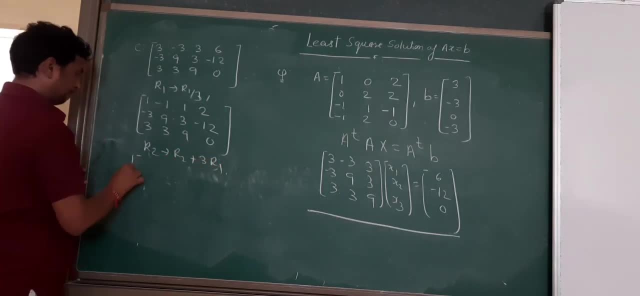 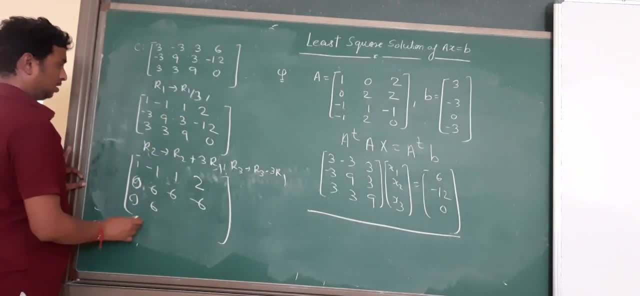 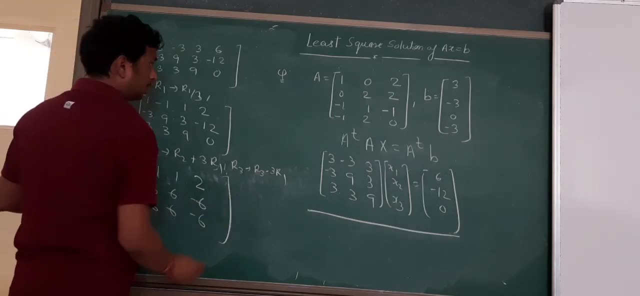 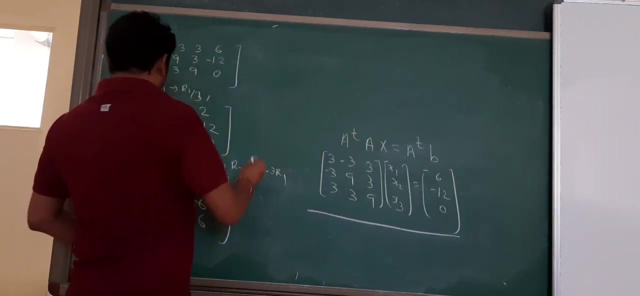 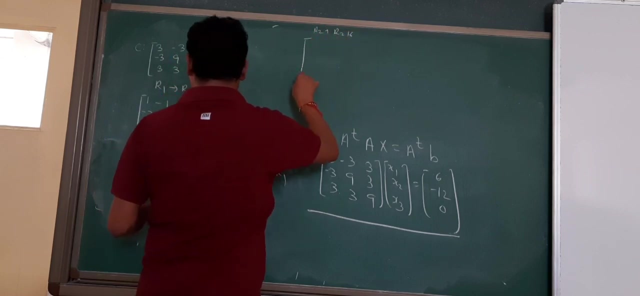 0, 6, 6, R3, 갈 hole 6, shovel 6 and the minus 6 is 0.. Guys, please Build in R2, R2 plus R3 minus 11.. R2 by 6, so what we get 1, minus 1, 1, 2, 0, 1, 2, 1, minus 1, 0, 6, 6, minus 6, then. 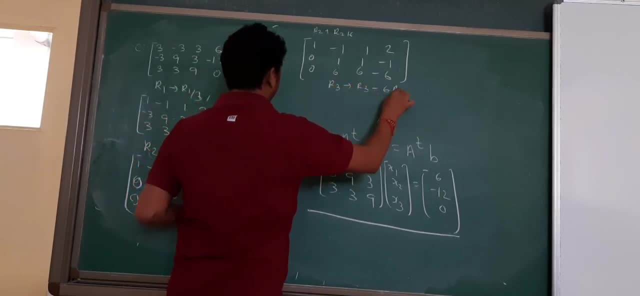 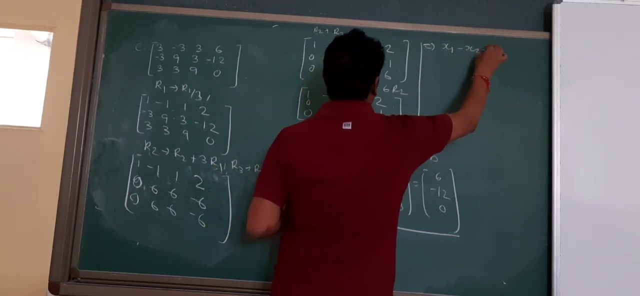 R2 by 6,, 1, minus 1, 1, 2, 6, 0,, 0,, 0,. so this is final matrix. so write it in equation form. it means x1 minus x2 plus x3 is equal to 2, then x2 plus x3 is equal to 2, then. 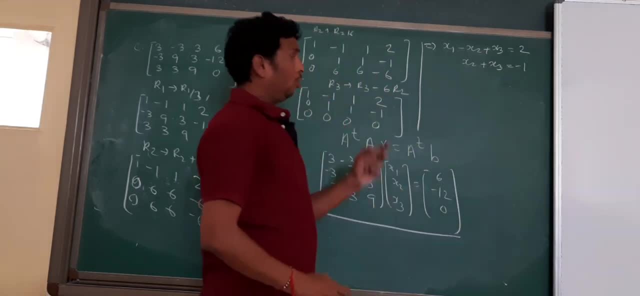 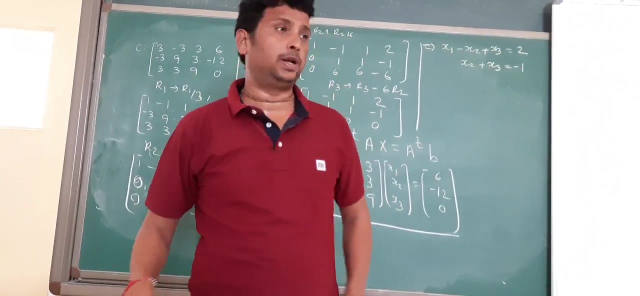 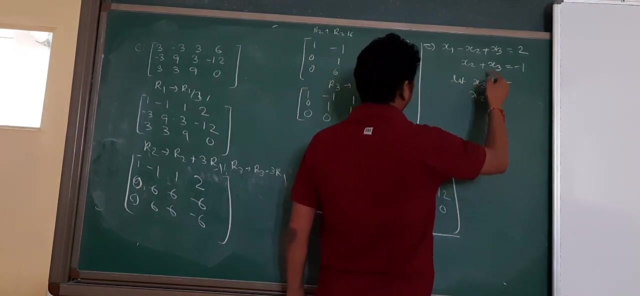 2 minus 1, and then 7,, only 2 equation and 2 equation 3: unknown. it means we have to consider 1 as a variable t. so let, x3 is t. what is x2, x2 is how? how much minus? 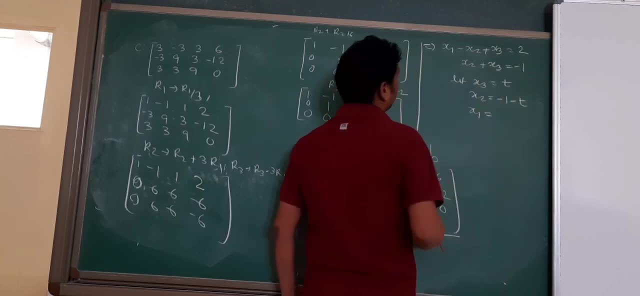 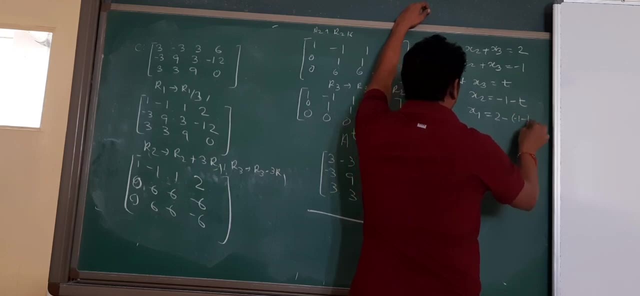 1, minus t. what is x1,. x1 is 2 minus xk, minus x2 means minus 1, minus 1, minus 1, minus t, minus x2, plus xk plus t. so how much 2 plus 1, plus 2t, correct, minus plus. 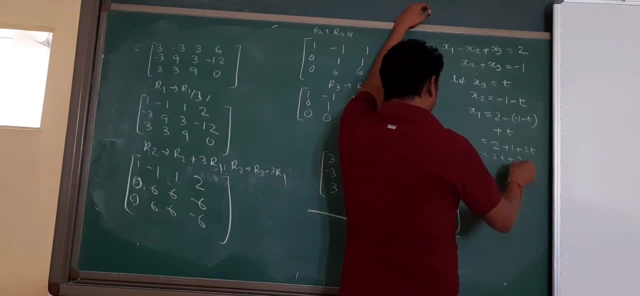 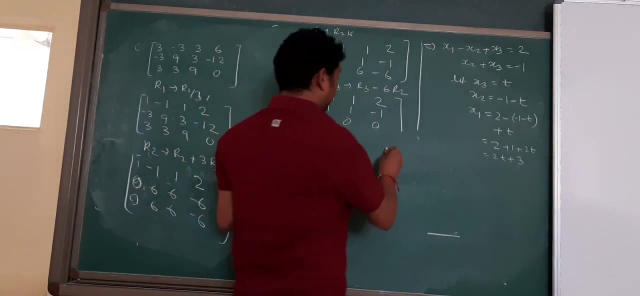 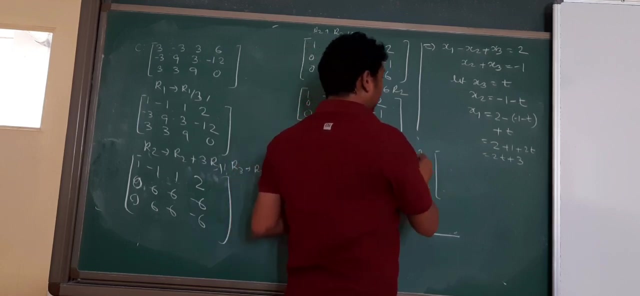 t, so 2t plus t. so it means what is the solution? solution is x, x is x1, x2, xc. and what is x1?? x1 is 2t plus 3, what is x2, minus t minus 1, what is xc? t plus 0, so this is the thing. 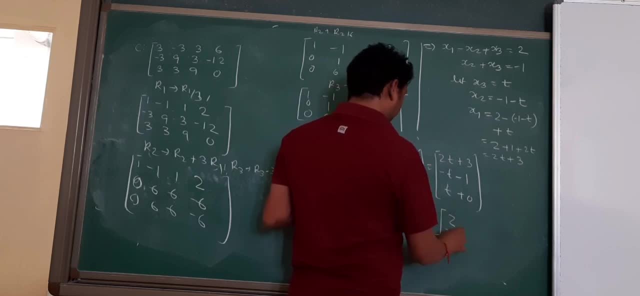 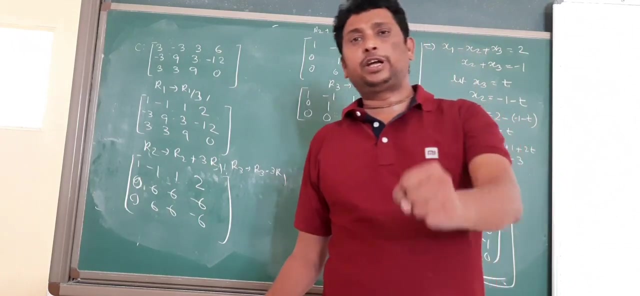 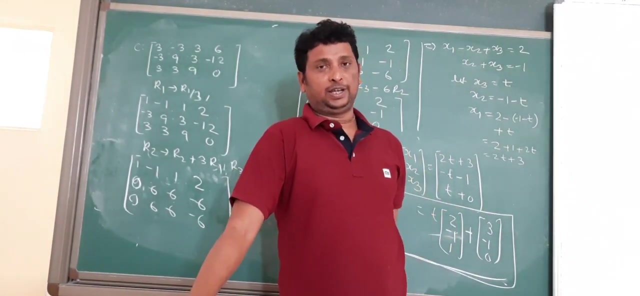 that we have to keep 1, 2, minus 1, 1, plus 3, minus 1, 0, so this is the solution of the system of equations. this is the least square solution which we obtained. hope you. 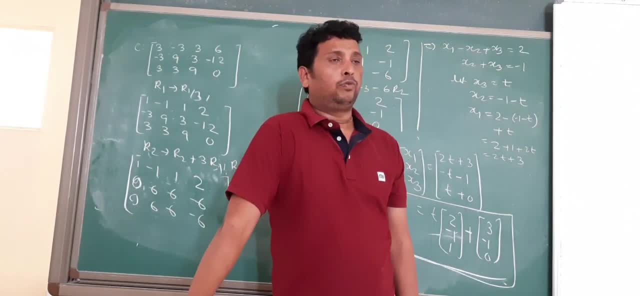 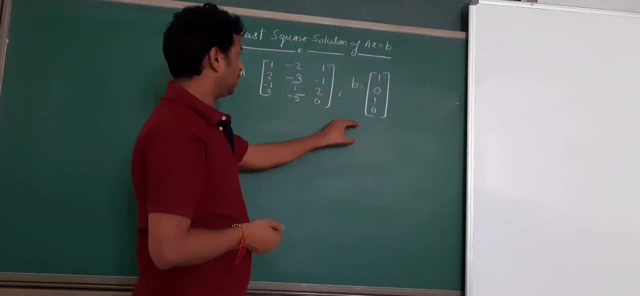 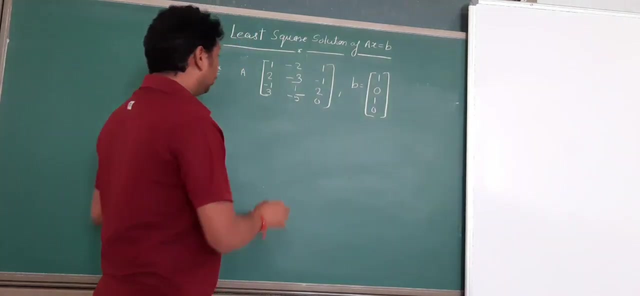 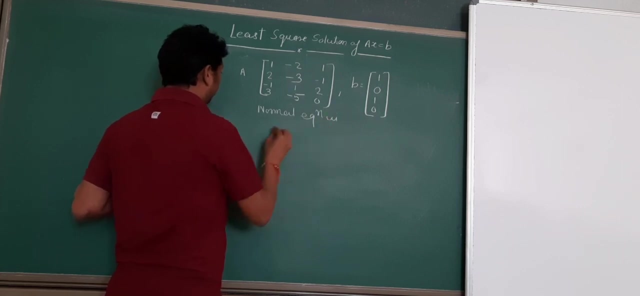 all understand this one. we do not all linear, least square solution, least square approximate solution of this system of equations. so how we find this is already written in matrix form, so just start. So we have to write the normal equation. the normal equation is, you know very well. 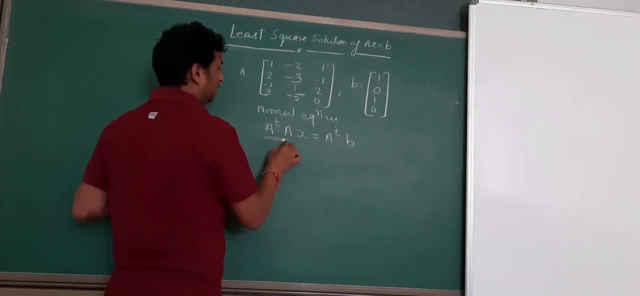 a transpose into a of x is equal to a transpose into b. it means we have to calculate first a transpose of a and a transpose of b. so what is a transpose into a? It is simple: first write a transpose. what is a transpose? 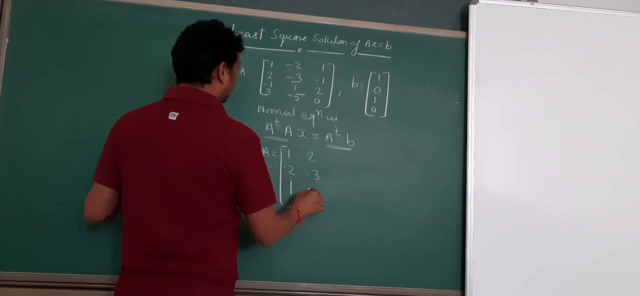 1 minus 2, 1, minus 2, 1, minus 1, minus 2, minus 2, minus 3, minus 3, minus 1, minus 2, minus 3, minus 1, minus 1, 1, 2, 3, minus 5, 0. 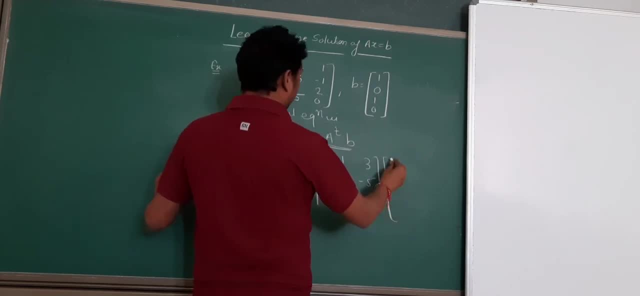 This is A transpose into A. A means 1, 2, minus 1, 3, minus 2, minus 3, 1, minus 5, 1, minus 1, 2, 0.. So now calculate A transpose into A. 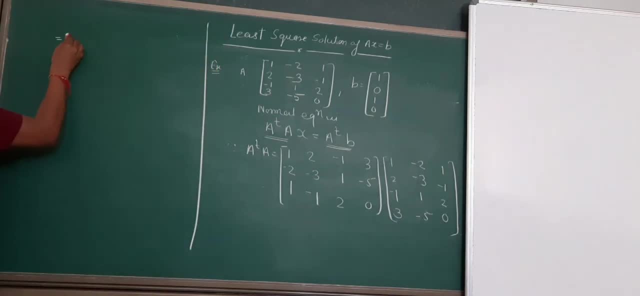 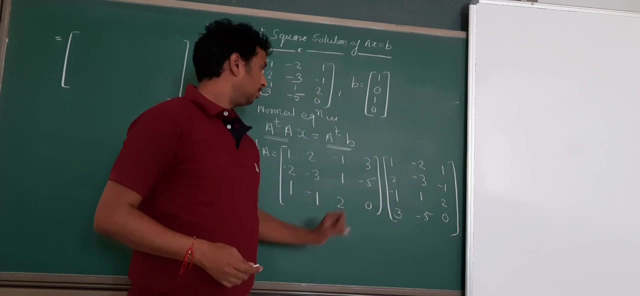 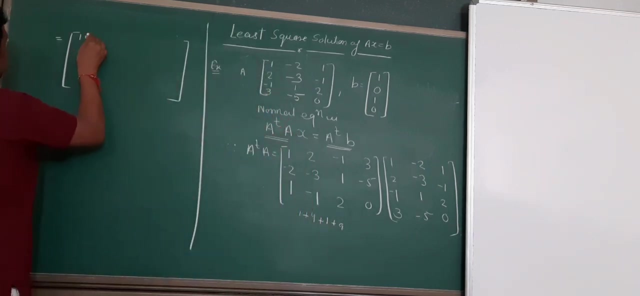 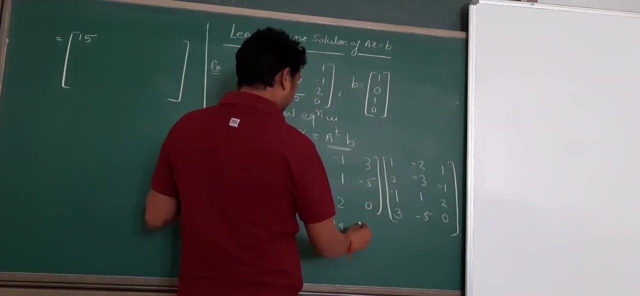 How to calculate Row into column. So what is first statement? 1 into 1.. 1 plus 4 plus 1 plus 9.. 50.. Then first row, second column. What is our answer? Minus 2, minus 6, minus 1, plus minus 15.. 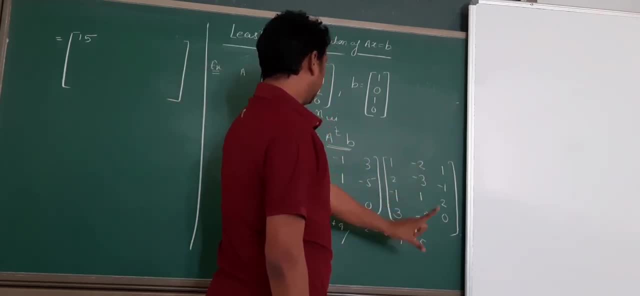 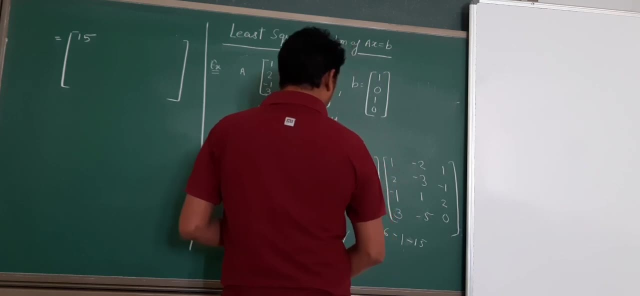 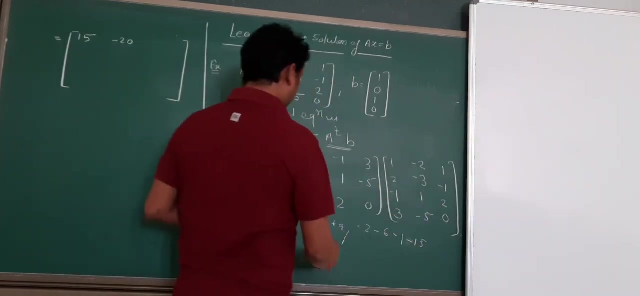 Minus 2, minus 6, minus 1, minus 15.. So total how much Minus 20.. So this is minus 20.. Then first into third: 1, minus 2, minus 2, 0.. 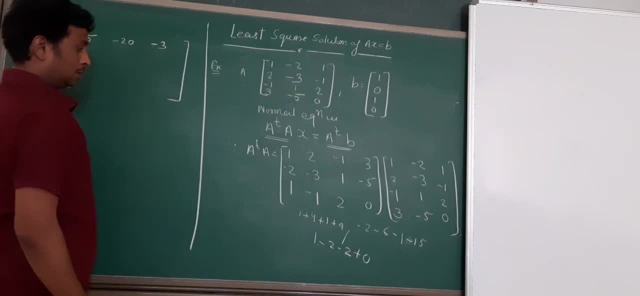 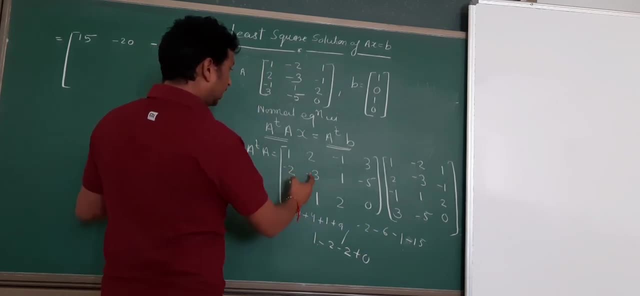 Minus 2.. Okay, Then for second Second row, first column. So minus 2, minus 6.. 1 into 3, minus 3, minus 6, minus 3, minus 15.. Minus 5.. 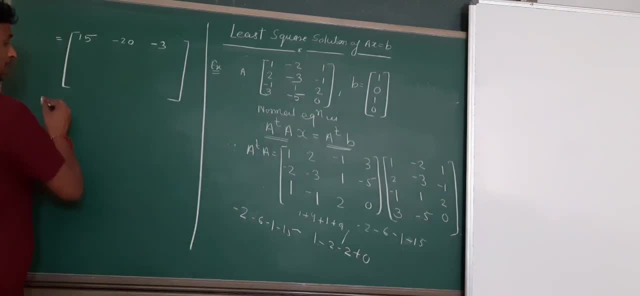 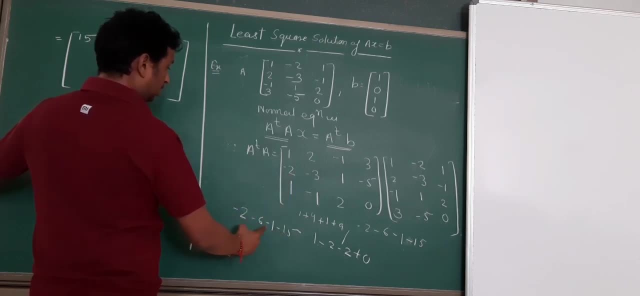 Then first row 1 into 3. That difference: 3 into 3. Minus 1. 1 into 3.. 2 into 2.. 4 into 5. Minus minus 2. 1 into 3.. 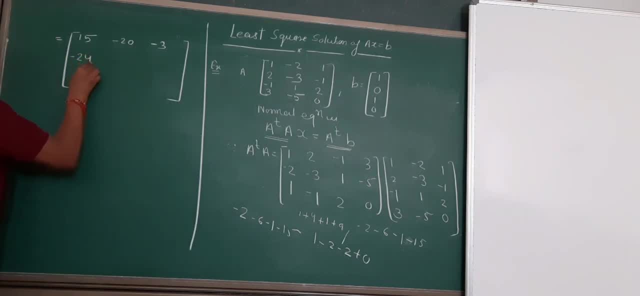 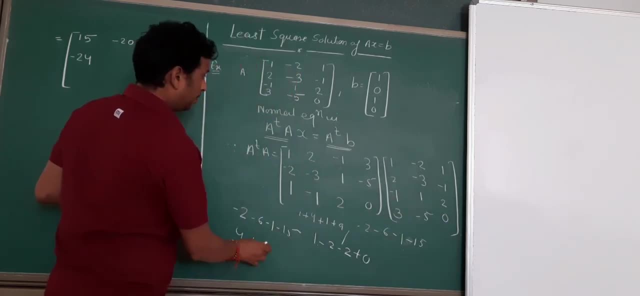 5 into 5. Minus 1. We get this 2 into 5.. Then 2 into 5.. 20 into 1.. 4.. 4, plus 9, plus 1, plus 25.. 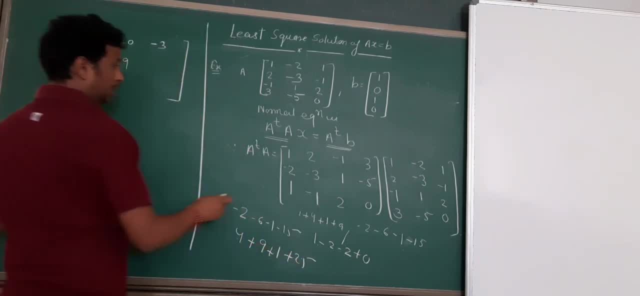 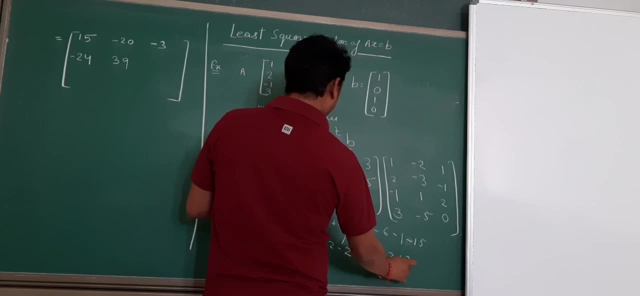 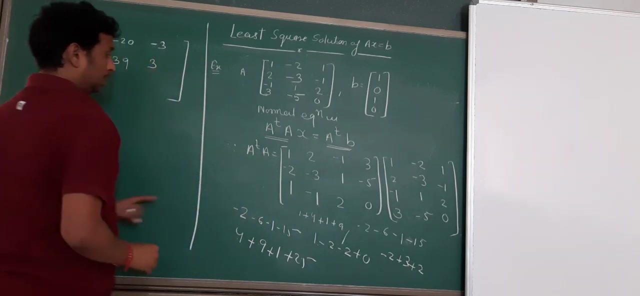 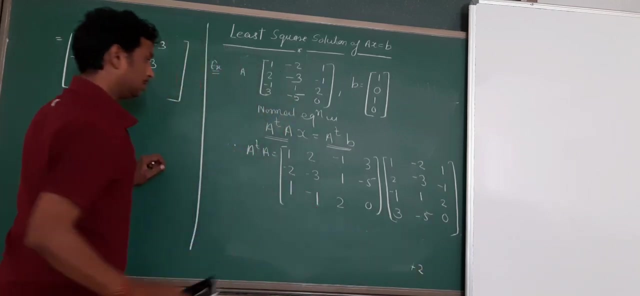 Very nice. Then second into third: Minus 2, plus 3, plus 2.. 3.. Then third into first. Third, into fourth: 1, minus 2, minus 1, minus 2.. Second into second. 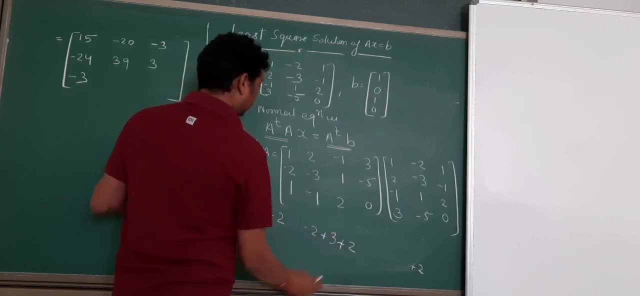 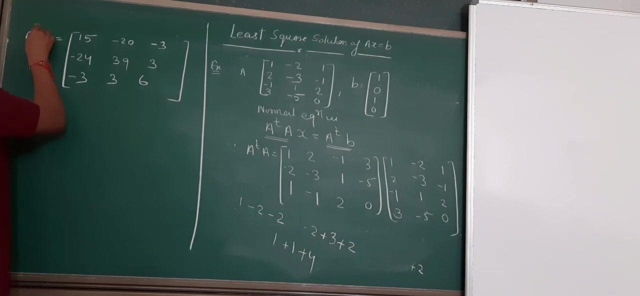 Minus 2, plus 3, plus 2.. 0. 3. Then third: 1, 1, plus 4, plus 4. 6. This is A transpose into A. Now we will complete. A transpose into B. 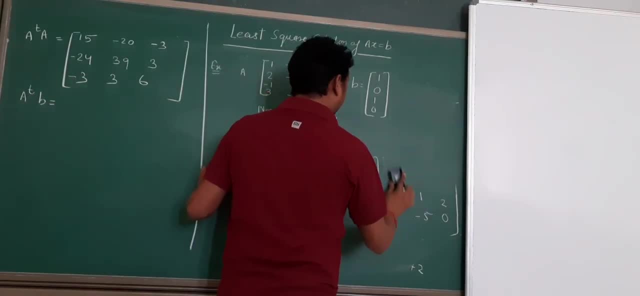 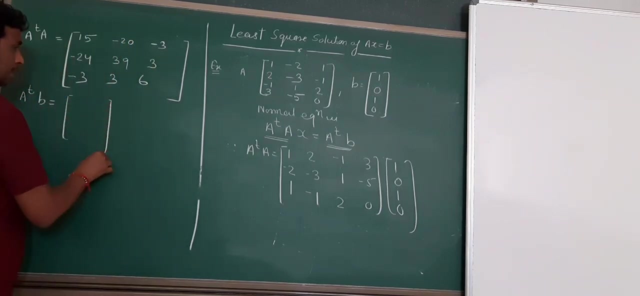 What will this A transpose into B? So write G matrix B is the same, B 1, 0,, 1, 2.. So first into second Again, it will be 1.. 1, minus 1, means 0.. 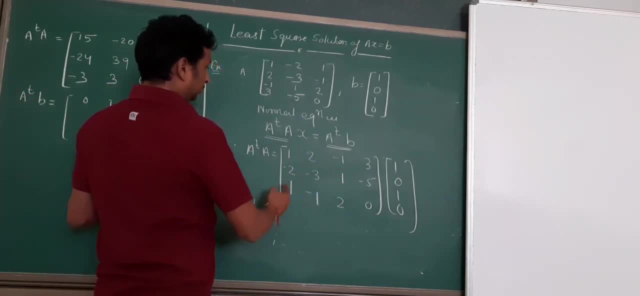 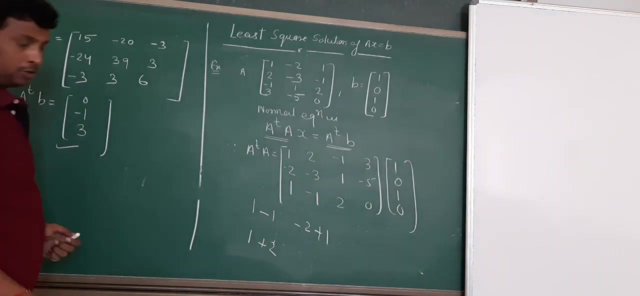 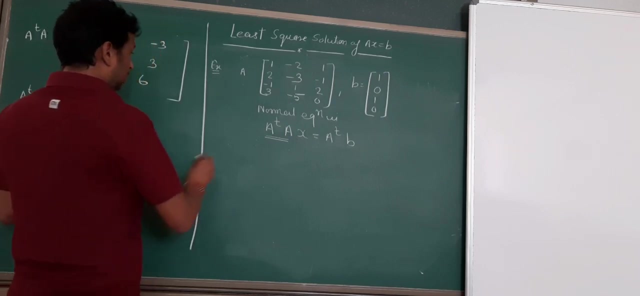 Starting with the first Minus: 2, 0, 1, 0. Minus 1.. Then third: 1, 0, plus 2, 3. This is unisys transpose into B. So it means what is normal equation? Normal equation becomes this way: 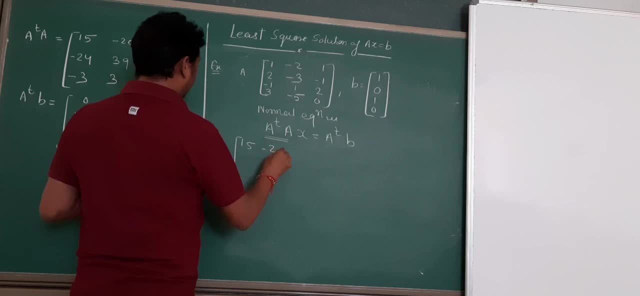 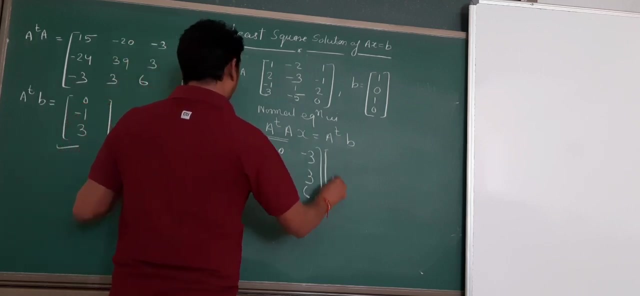 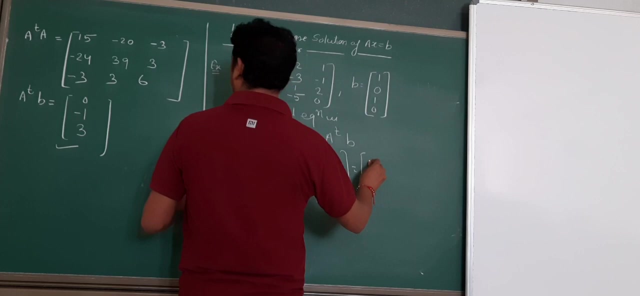 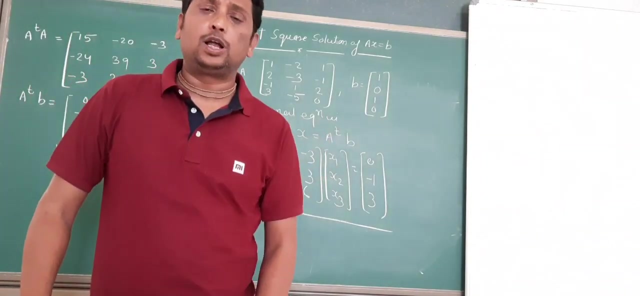 x1, x2, x3 is equal to A. transpose into B is 0, minus 1, 3.. So this is the final system of normal equation. Now we have to solve this one. That's all. So how we solve this one. 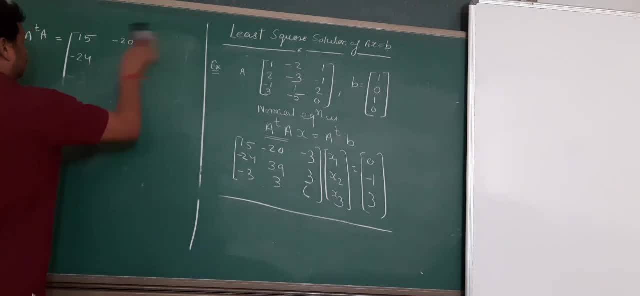 You know, in Gauss elimination method, first we have to say we want to do. we write: see augmented matrix. what is that? See augmented matrix. 15 minus 0.. What is that? 15 minus 0.. 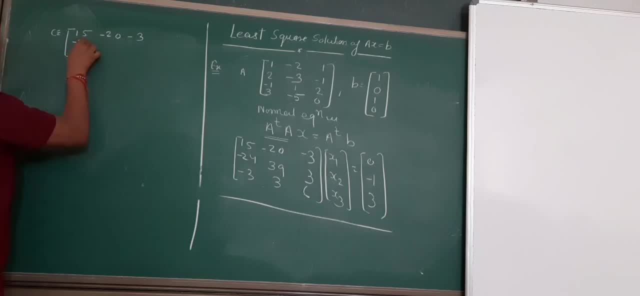 What is that? 20 minus 3, minus 24,, 39, 3, minus 3,, 3, 6.. And what is B 0, minus 1, 3.. So we have to reduce this one in an upper climate matrix form. 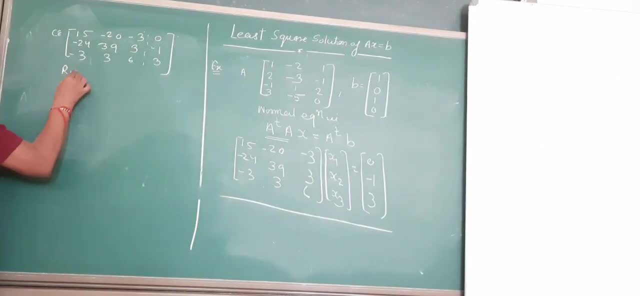 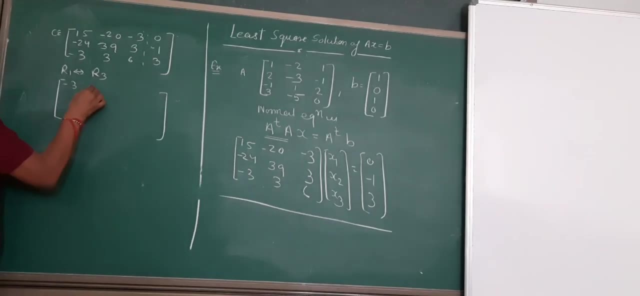 How we do. First we change the row means R1 being touched with R3.. So what do we get? Minus 3, 3.. 6, 3.. Second same same: 15 minus 20, minus 8, 0.. 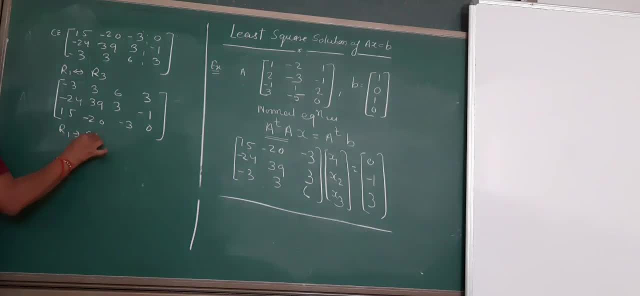 Then R1 divided by R1 by 3. What do we get? Minus 1.. Minus 1.. Minus 2, minus 1. This is same. Minus 2. Minus 3.. 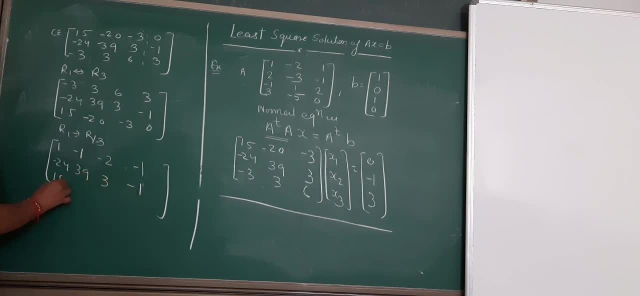 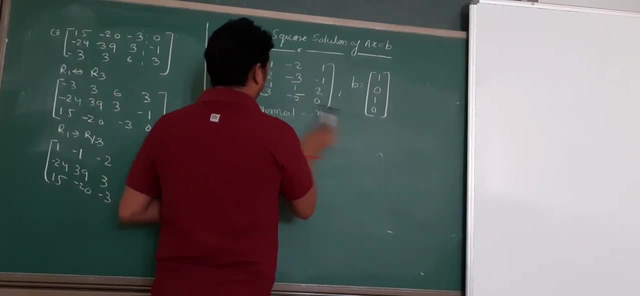 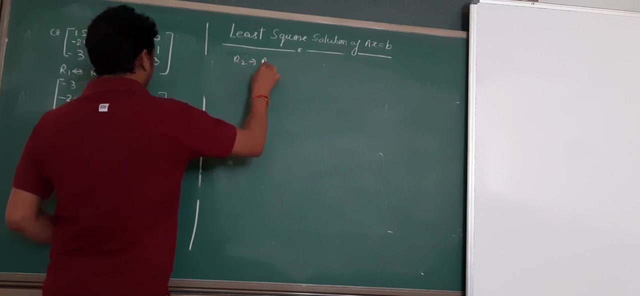 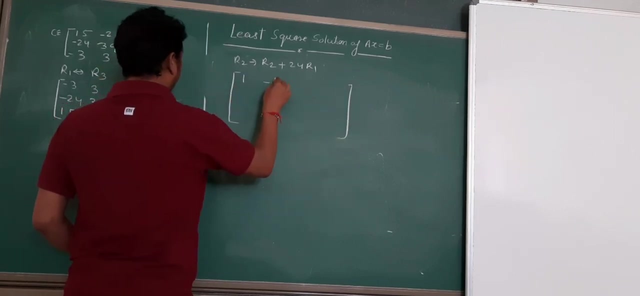 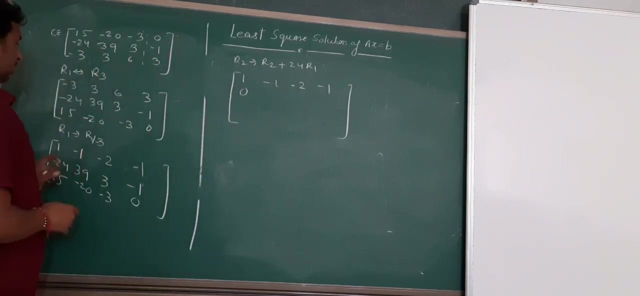 this is z. then make cos element below 1,, 0,. how we get 0,. so r2. change to r2 plus 24, r1,. what we get: 1, minus 1, minus 2, minus 1,. this is 0,, 24,, 39,, 24,, 15, so minus 24. 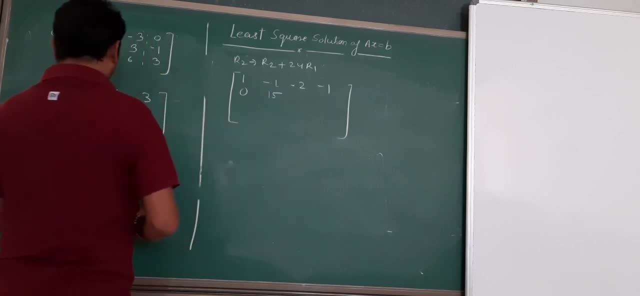 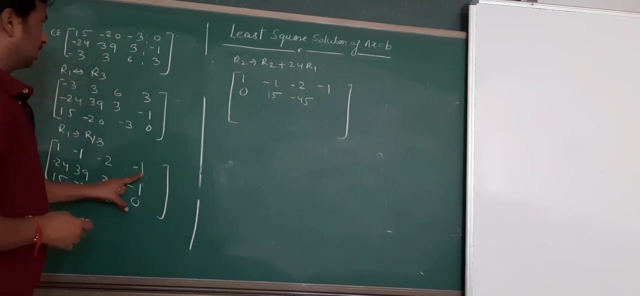 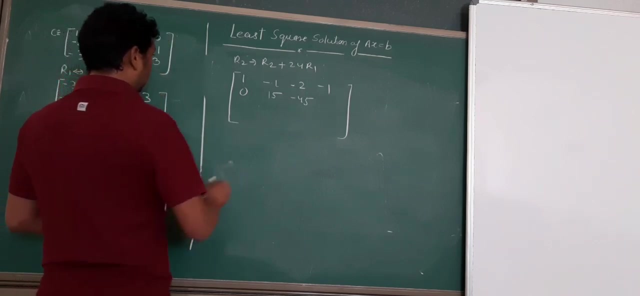 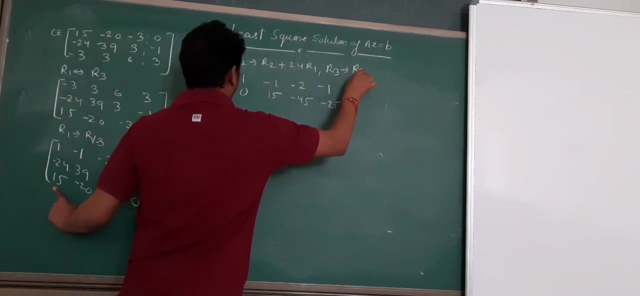 plus r1,. okay, 24 means minus 28,, 48, plus 3.. minus 45,, 24, minus 24, minus 25, this one also becomes 0,. r3. change to r3 times 15,. 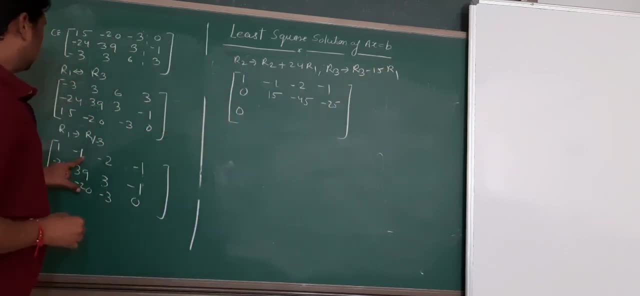 r1, so this is 0, 15, minus 15, plus minus 20, plus 15, means 5, minus 5, this is 0, here minus 20, minus. when you multiply with z, that is correct, are we doing minus. 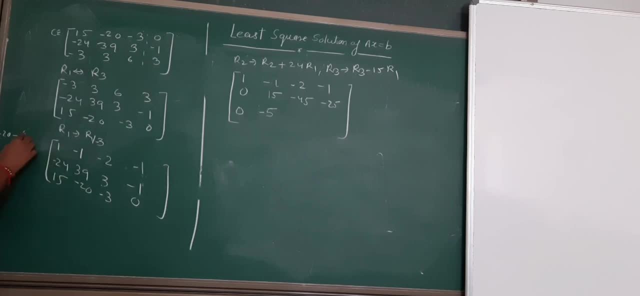 15, here plus 15,, so this is 10,. this is the gradient, okay, so how we do: minus 15,, minus 15,, 10, plus 15,. okay, What is z? what is the value? 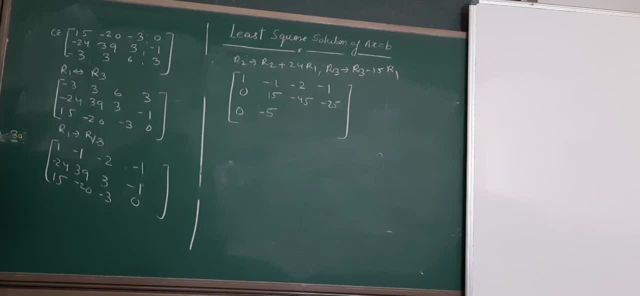 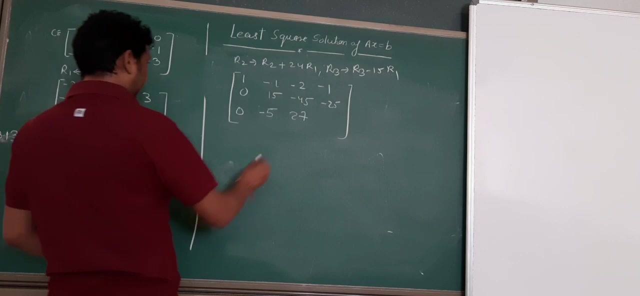 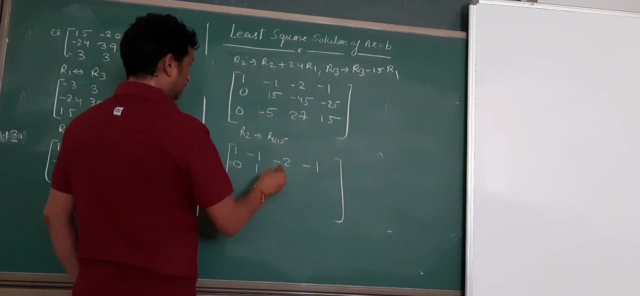 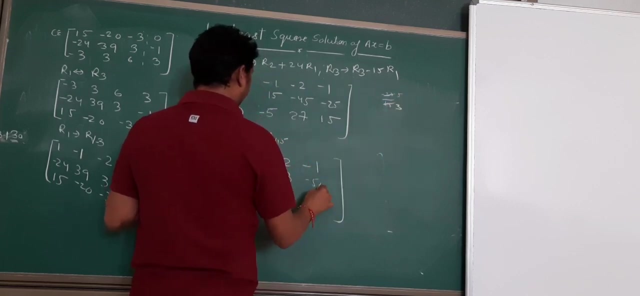 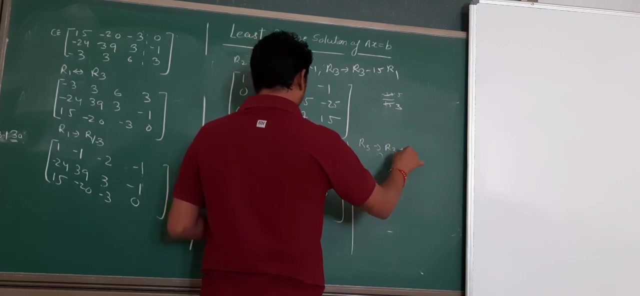 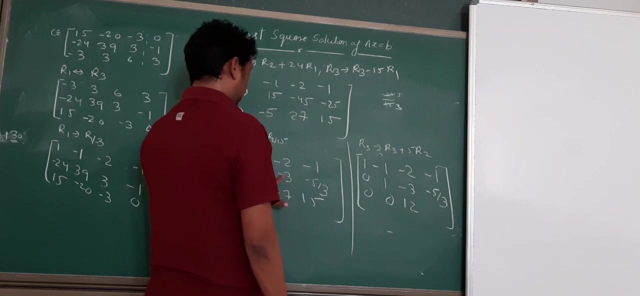 minus 30.. So I will make 1 divide R2 by R2 by 15.. 1 divide R2 by R2 by 15.. 1 divide R2 by 15.. 1 divide R2 by 15.. 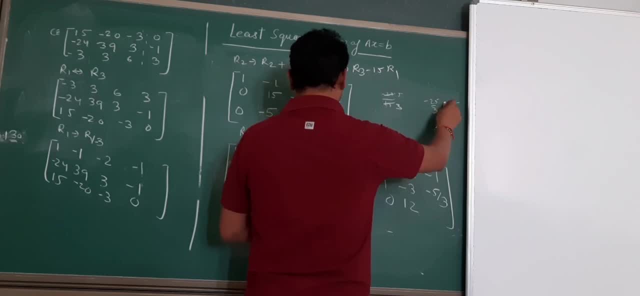 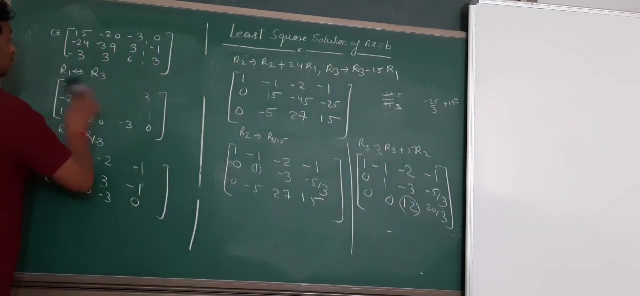 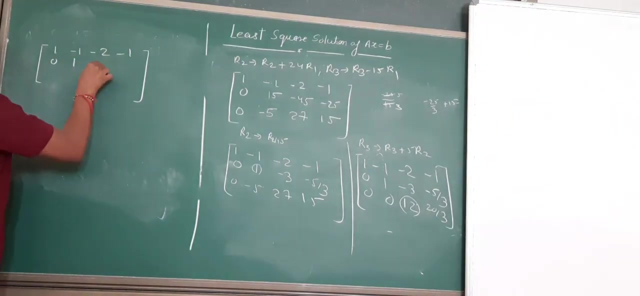 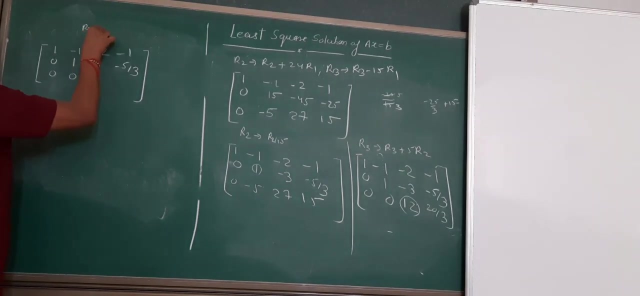 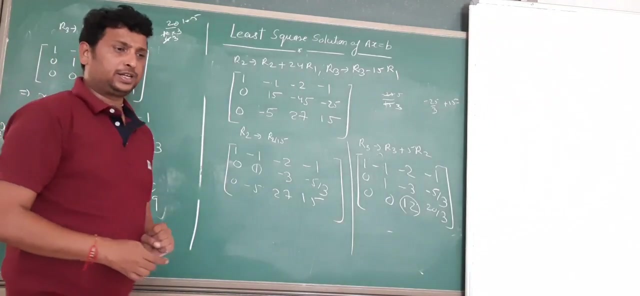 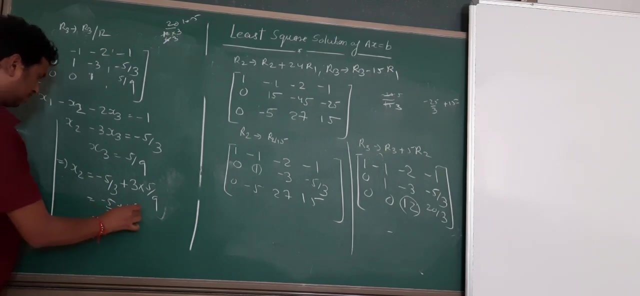 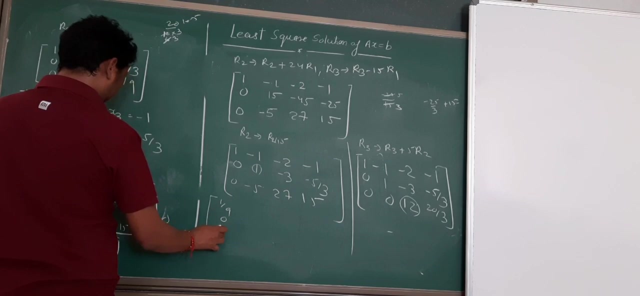 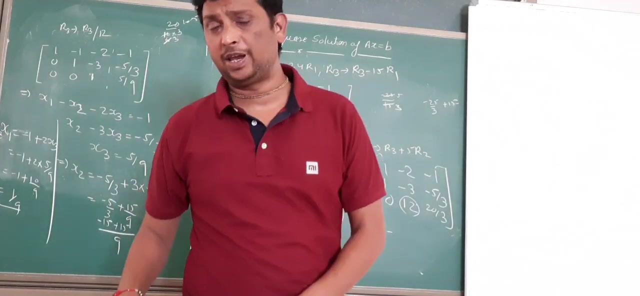 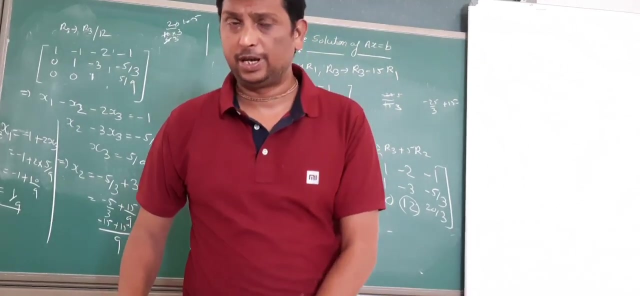 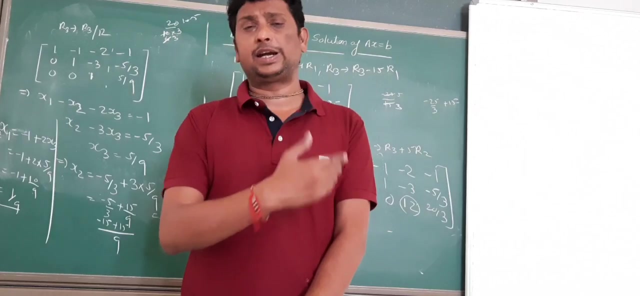